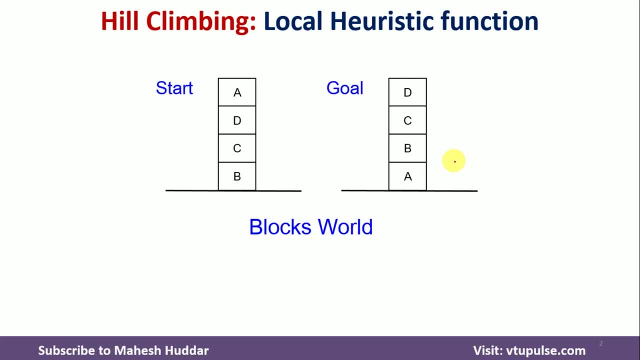 function and where we will consider the global information, or you can say that what will happen in future? based on that we will select the operator where we can go from a start state to goal state here. so first we will consider the local heuristic function. in this local heuristic function we will give plus one. 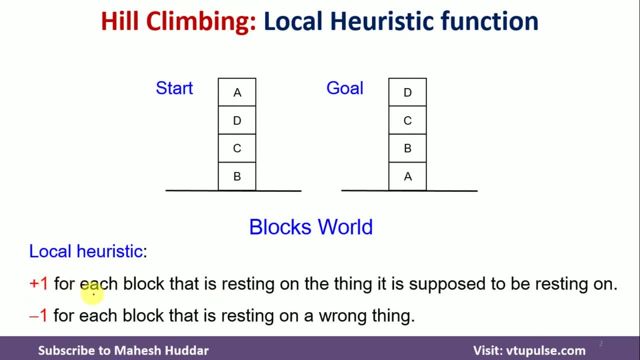 reward for each block that is resting on a thing it is supposed to be resting on. that is, for example, we are expecting B should rest on a, a should rest on ground. similarly, C should rest on B, D should rest on C. if it is the case, we will give. 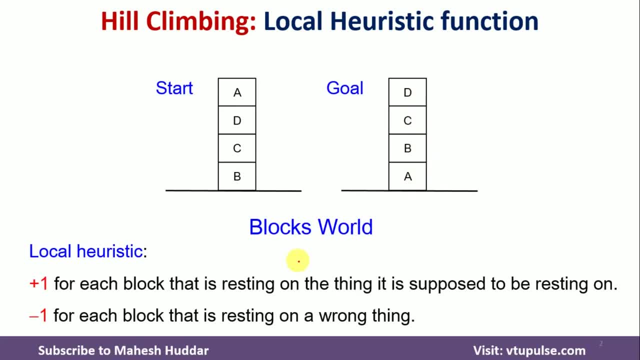 plus one if anything else is there, for example, in this particular start state only, and B is present on a ground. but what we are expecting a should be present on the ground, so it will be given as a minus one. we are expecting C should be present on B. yes, it is present, so it will be given as a plus one, and so 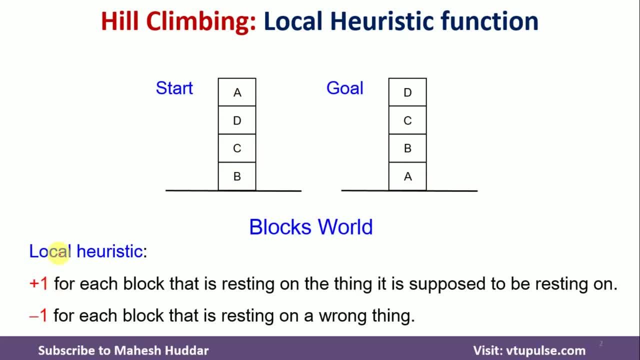 on. so that is what the local you information or a local heuristic function here. so we will try to calculate what is the value for the start state. the start state is it will be minus one because it is not present at the correct position here. for C, C is. 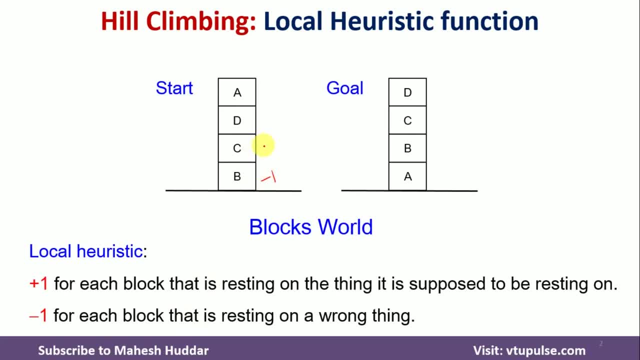 expected to be present on B, and it is present, so it will be plus one. this is also plus one, but this is minus one, so the total value of this particular start state is zero here. now, when it comes to goal state, all of them are present on the 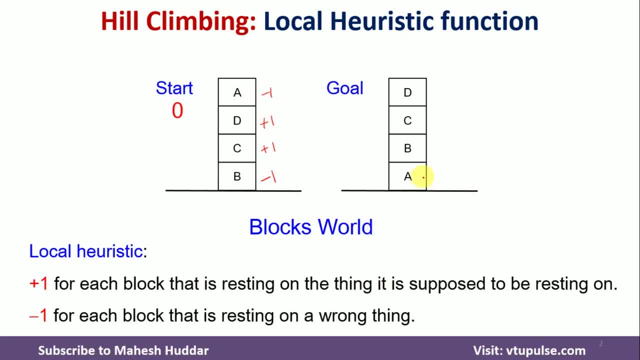 current position. of course they are present on the correct position. so everything will be given as you can say that plus one over here. so the answer or the value of this particular function is you can say that the plus four here. now, using this particular local information, we have to go from start state to goal. 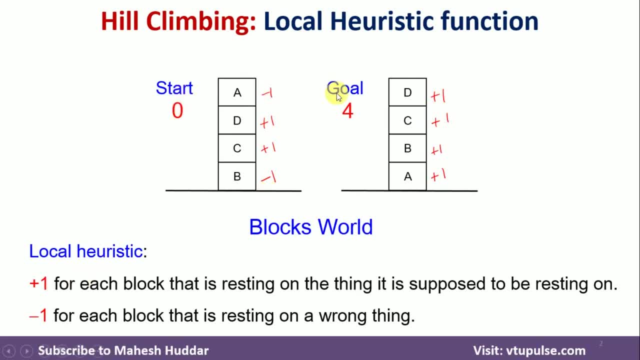 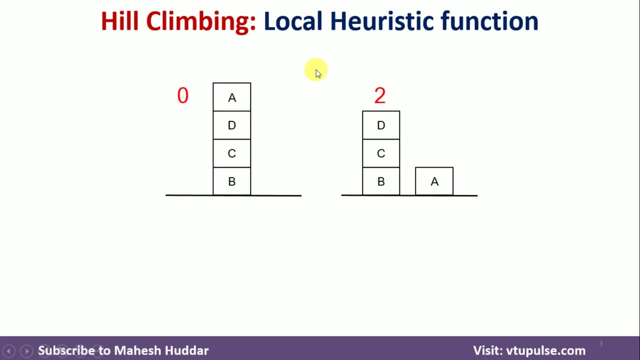 state over here. now we have to apply some different operators at the start set so that we can go to the goal state here. so first operator is: I will bring this particular A to the ground. so that is the only option. what we have here now. B is present on the ground. that is incorrect position, so it will be minus. 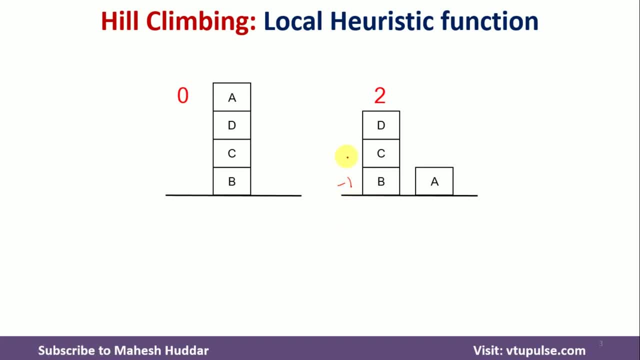 one. C is present at the correct position, D is present at the correct position, so this will be given as a plus one here. A is present at what we can say that the correct position, so it will be given as the plus one. now, if I add everything, I 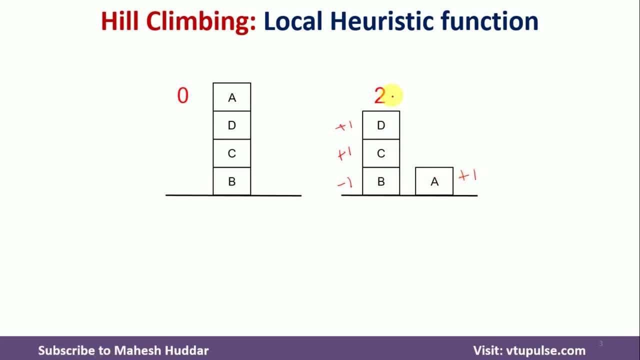 will get the plus two as the answer in this case. now there are two possibilities. are there? either I can move this particular D to this on the top of A, or I can move this particular D to this particular ground now, if I do this particular operator, if 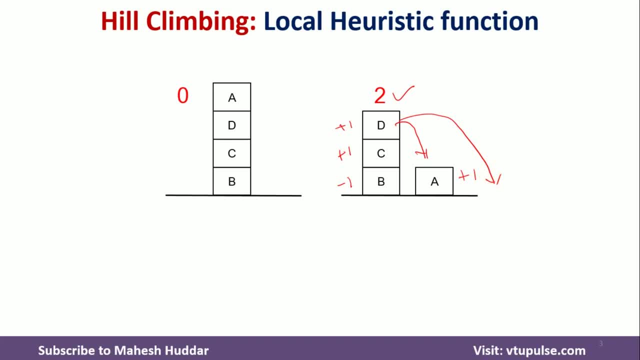 I apply this particular operator. what will happen? we will try to see. if I move this particular D on the top of A, I will get the value as 0, and if I move this particular D to the ground, I am getting the value as 0. why? because B is. 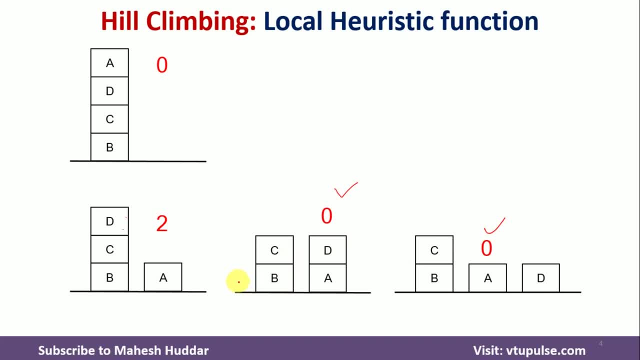 incorrectly placed. D is incorrectly placed, a and c are correctly placed here, so the value is zero. similarly, c is correctly placed here, a is correctly placed, b and d are incorrectly placed. so because of that, we are getting zero here. because we are getting zero, zero in both the cases, we have ended up with something called as. 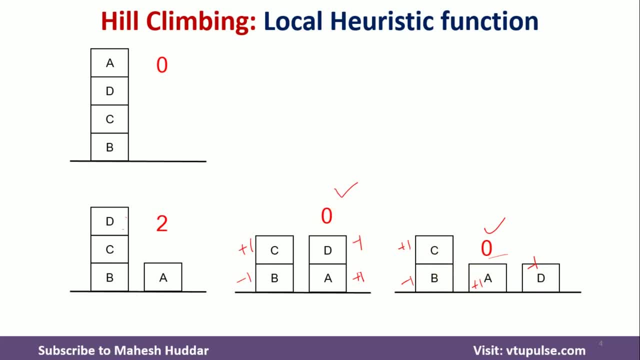 the local maximum, or can say that a local optimum. okay, so because of this, we cannot go ahead from here onwards. this is the disadvantage of using a local heuristic function or a local information. i'm not able to reach what you can say that the goal state using this function, so what i do is i: 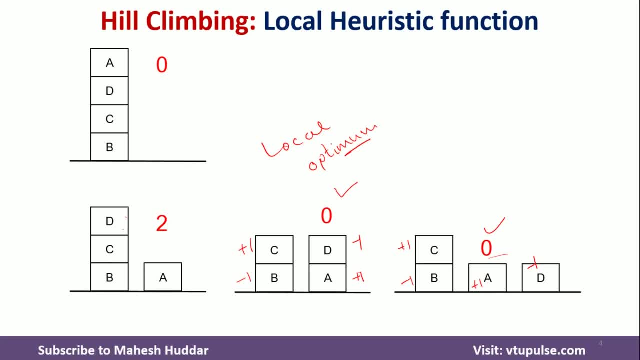 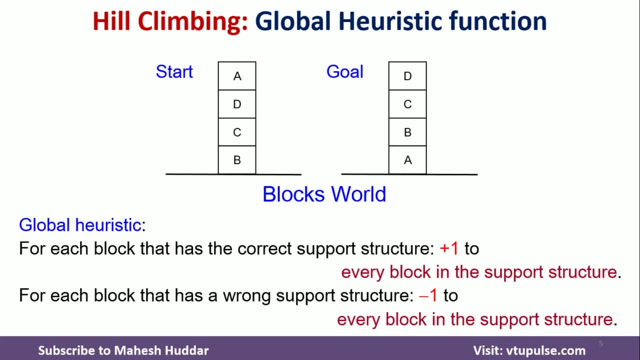 will use an global information or a global heuristic function. we will try to see whether i will be able to go from the start state to goal state or not. so in this case, again, the start state and the goal states are same, but the heuristic function is something like this: 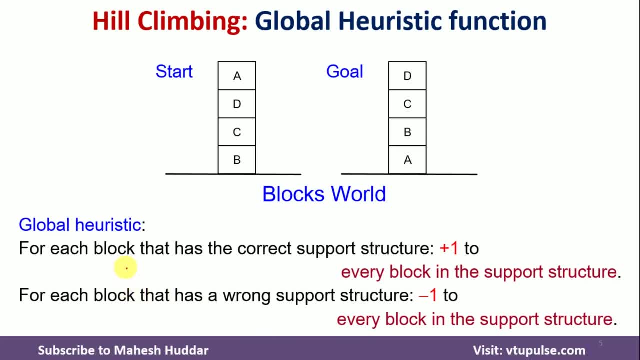 so in this case again, the start state and the goal states are same, but the heuristic function is: for each block that has the correct support structure, the plus one will be given as a reward for each, for every block. you can say, for each block that has a wrong support structure. 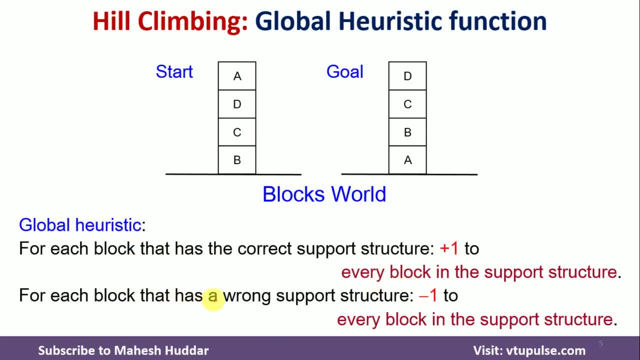 a minus one will be given support structure in the sense, the blocks which are present below the current block. if, if all of them are correctly placed, one will be given for every block. actually, if they are not correctly placed, minus one will be given for every block again. 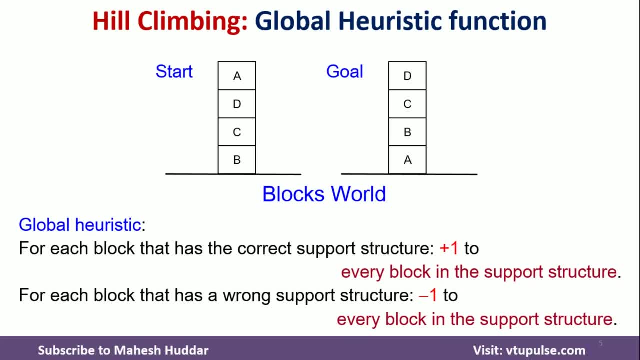 okay, so you can see here, below b we don't have anything, so it will be zero. but below c, b is present. whether b is present, the correct position. no, so it will be minus one below d, c and b are there? both of them are correctly placed. no, they are not correctly placed, so it. 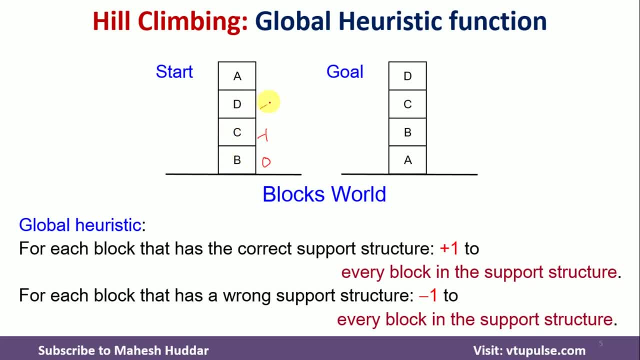 will be minus two. below a, b, c, d, are there? all of them are not correctly placed with respect to the goal state, so it will be minus three. so the total value of this particular block is minus one. so the total value of this particular state is minus six. now coming back to this goal state. 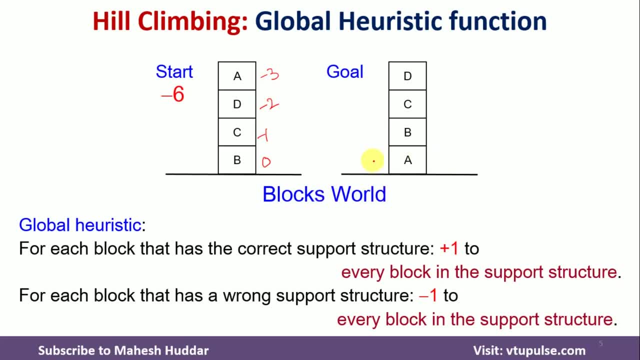 of course all of them are present at the correct position. so below a we don't have anything, so it is zero. below b we have one node, so it will be one here. for this one it will be two, for this one, it will be three here, because below d three nodes are there, or the three blocks are there, all of. 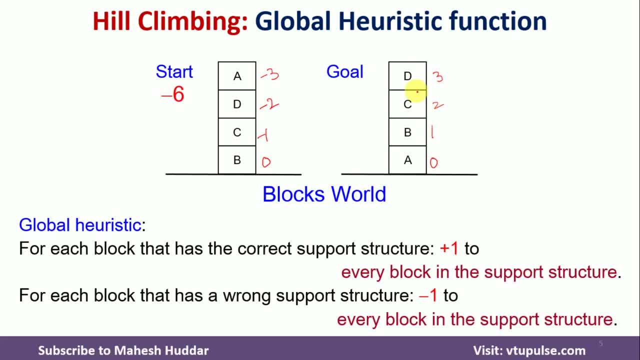 them are correctly placed here, so it is plus six. so the intention is to go back to this goal state from start state to goal state that is minus six to plus six here by applying different operators. so what i do here is first i will move this particular a to this particular ground. now, if 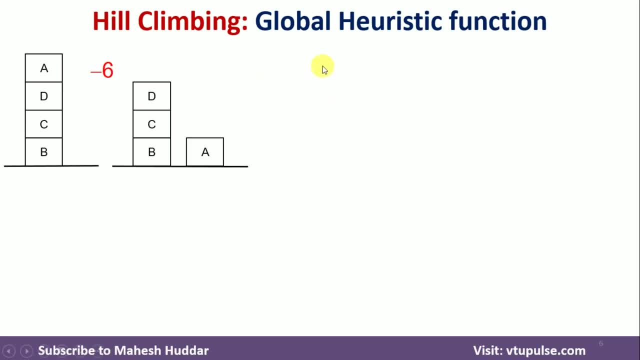 i move this particular a to the ground b. below b: we don't have anything, so it is zero. below c: b is present. it is incorrectly placed below d. we have c and b. both of them are incorrectly placed below a. we don't have anything, so it is zero. so the total value of this state is minus three. 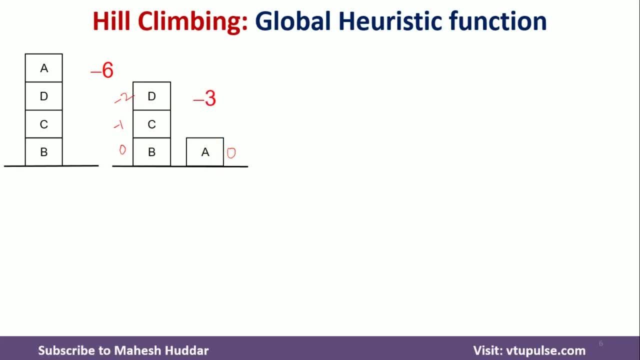 now there are two possibilities are there? either i can move d on the ground or d on the top of a, and now i will move this particular d on the ground. i will see what will happen now. if i move d on the ground, this one will be zero below c. we have one block. that is incorrectly. 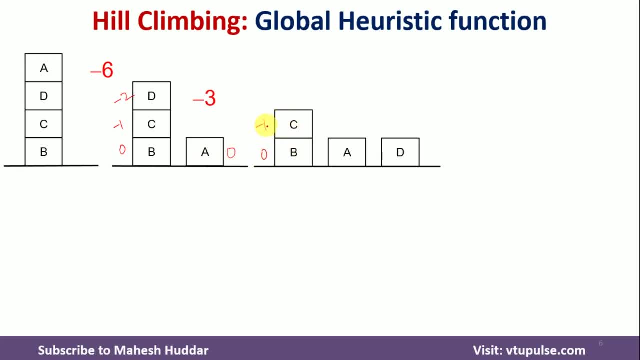 placed below a, we don't have anything, so it is zero. below d, we don't have anything, hence it is zero. so the total value of this particular state is minus one. so it is better than the previous one. so we will consider this one here. now i will move c on the ground. it will look something like this: all of them are not correctly. 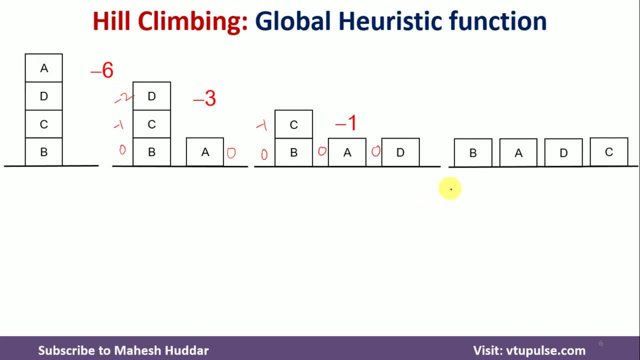 placed, but below this particular thing the support structure is not present. so all of them are having 0, 0 as the value. so the value of this particular state is 0. again, it is better than the previous one. so i will continue from here onwards. now i will put b on the top of a here. so if i put b on 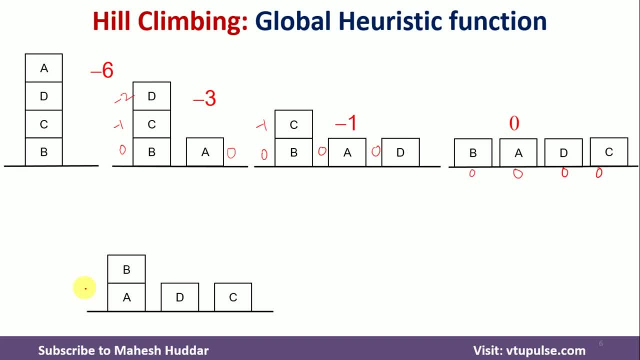 the top of a, for a it is 0, because below a we don't have anything, below b we have 1- can say that the block which is correctly placed- hence it is plus 1, and then for d it is 0, for c it is 0. 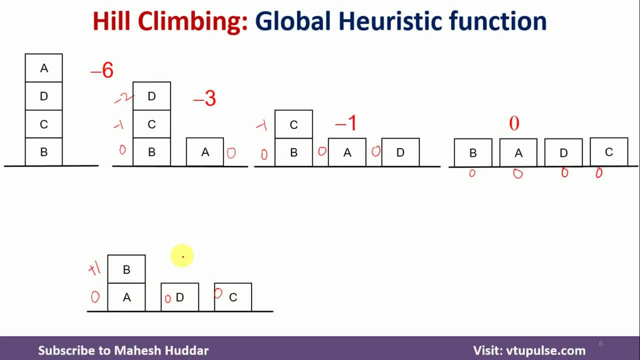 so the total value of this state is 1 here now i will move c on the top of b. below a we don't have anything. that's the reason it is 0. below b, we have one block, and it is correct. and below a we don't have anything. that's the reason it is 0. below b, we have 1 block, and it is correct. 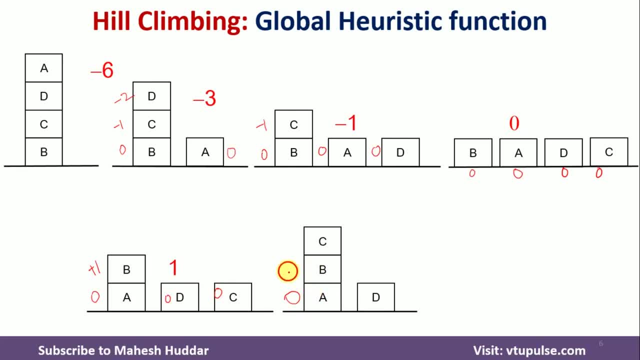 correctly placed, so it is 1 below C. we have two blocks, A and B. both of them are correctly placed. it is 2 below D. we don't have anything, so it is 0. so the total value of this particular state is 3 in this case. now coming back to the last one, that is, move D on the top of C. all of them are. 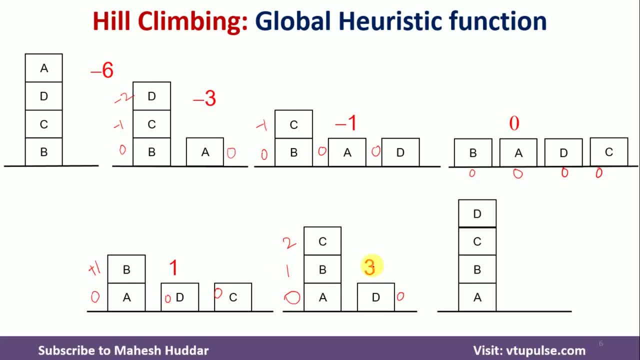 correctly placed. for A it is 0. for B it is 1, because one correctly block is present below B, below C, we have two blocks. both of them are correctly placed. below D we have three blocks. all three blocks are correctly placed here, so the total value of this particular state is equivalent. 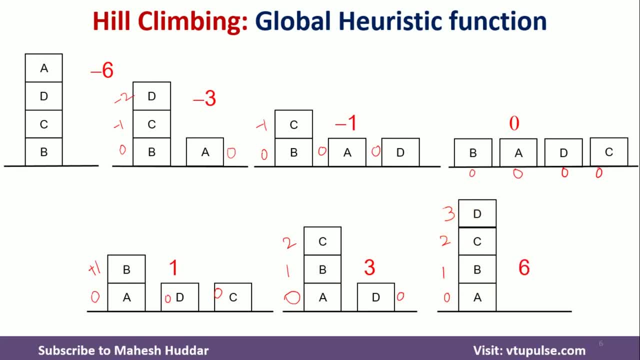 to plus 6. so we started with minus 6, we ended up with plus 6, using this particular global heuristic function in this case. so this is how actually we can use either local or global heuristic function to go from initial state to goal state using hill climbing algorithm. 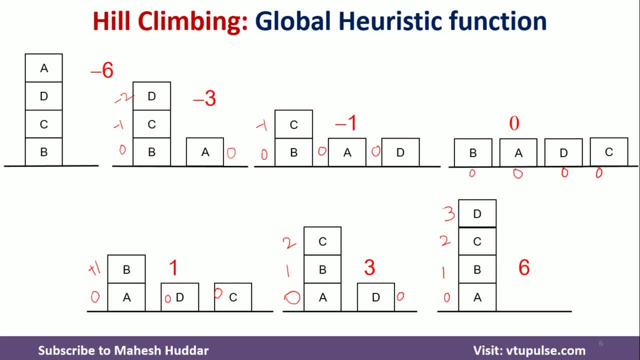 so this is how actually we can use either local or global heuristic function to go from initial state to goal state. I hope this particular concept is clear. if you like the video, do like and share with your friends. press the subscribe button. for more videos, press the bell icon.